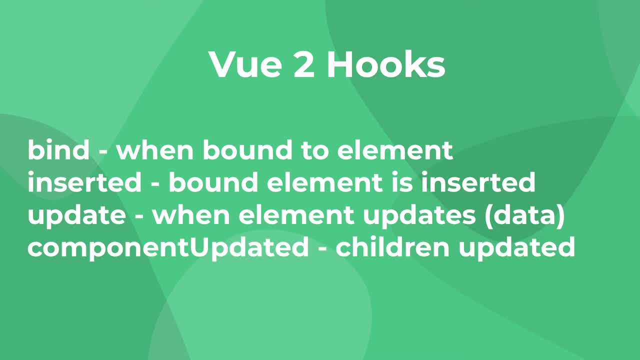 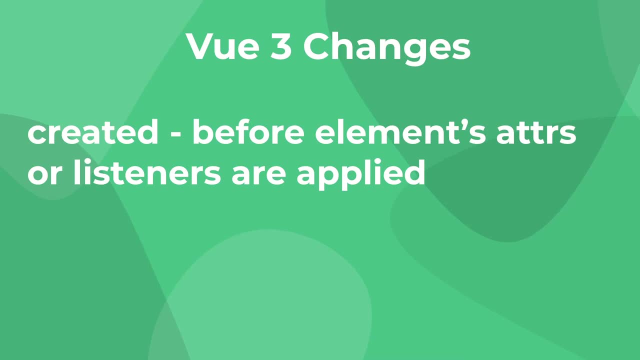 component updated, which is called after those children have updated, and unbind, which was called once the directive is unbound from an element. Vue 3 renames these hooks and adds some new ones. It adds a created hook, which is called before the element's attributes or event. 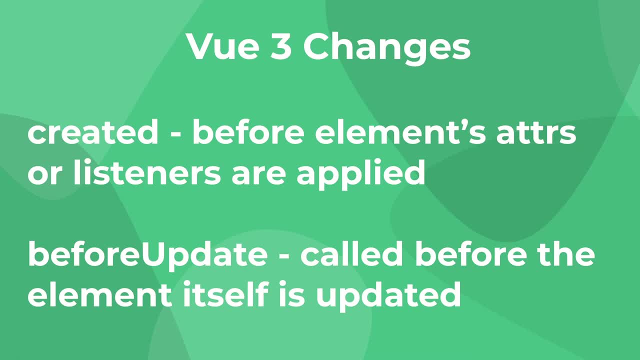 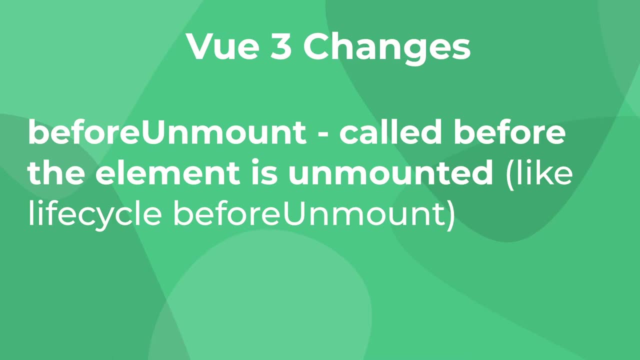 listeners are applied A before update hook, which is called before the element itself is updated, Kind of like a lifecycle hook. Then, finally, it adds a before unmount hook, which, again like lifecycle hooks, is called before an element is unmounted. So, regardless if you're working in Vue2 or Vue3, when you implement these hooks, 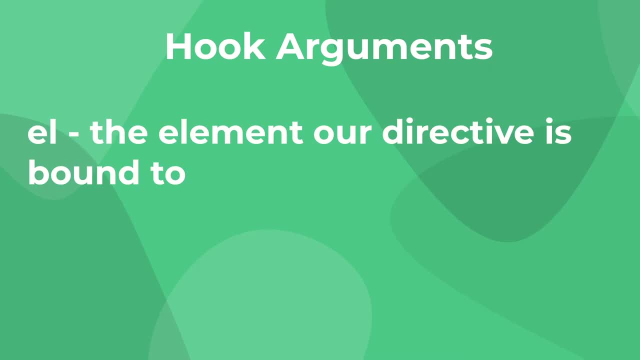 they accept the same argument, l, which is the element that this directive is bound to, and it gives you access to modify its CSS properties, content or things like that, Binding, which is an object that contains a lot of properties that affect how our directive runs. 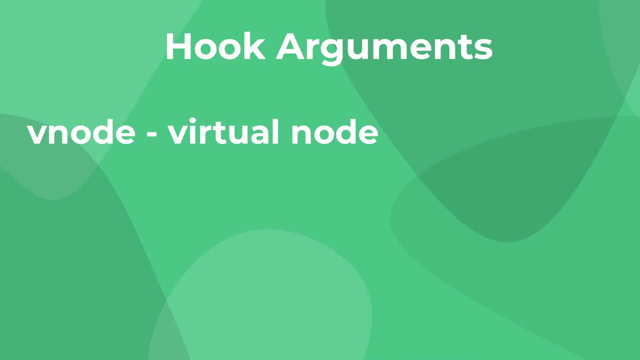 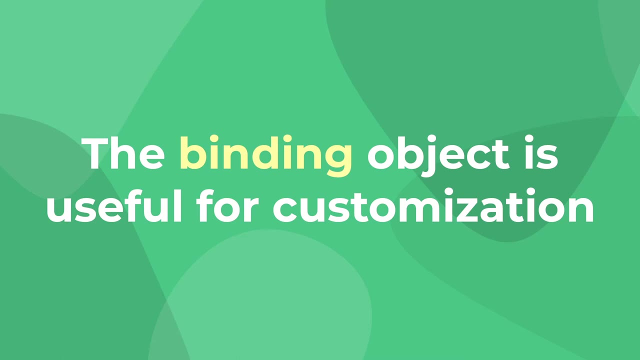 and we're going to go into depth in just a second VNode, the virtual node, and then prevVNode, which is the previous virtual node. So more on that binding object. The binding object contains several properties that will help you actually add functionality to your hooks. It has a name. 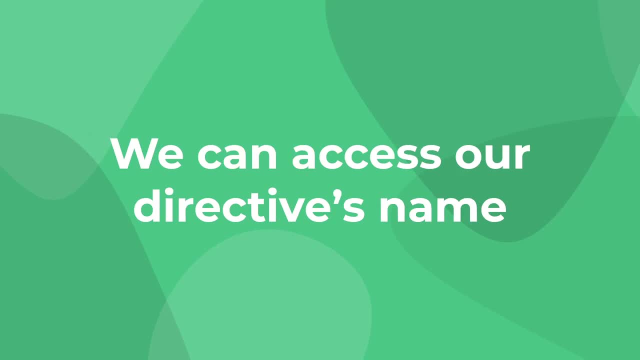 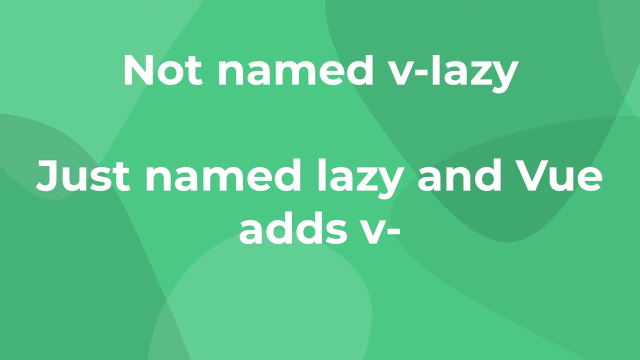 which is the name of your directive, without the v prefix. So, as we'll see in just a second, when you actually create your directive, it doesn't come like v lazy, it's just called lazy, and Vue will automatically add the v prefix. Binding contains the value, which is the value. 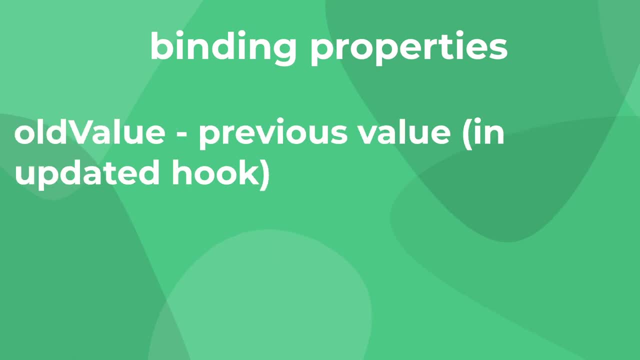 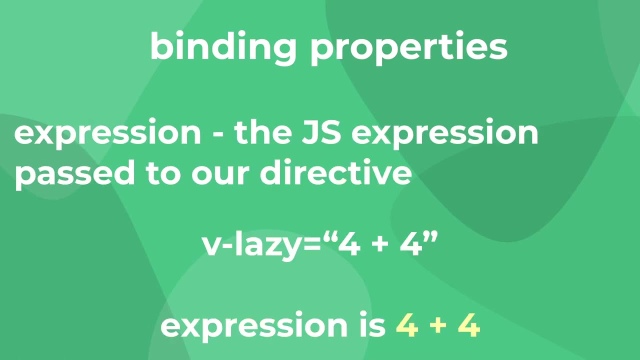 passed to your directive using a JavaScript expression: Old value, which is the previous value of directive, and this is available in the update. hook Expression is the entire expression that is bound to the string, So not just the value but the actual expression string itself. 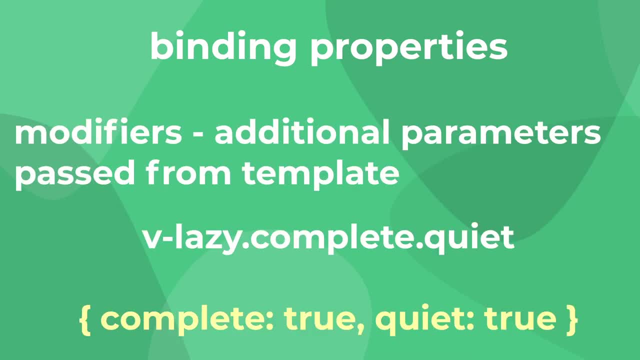 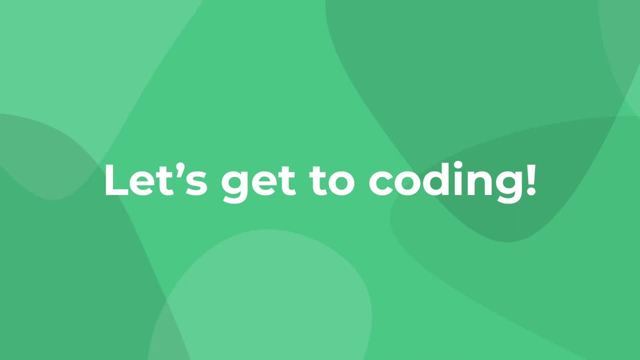 Arg, which is an argument passed with a colon, And then modifiers, and these are all of the modifiers inside a single object, And we can add multiple modifiers like this. Alright, so let's start coding, But before we move on, make sure to hit. 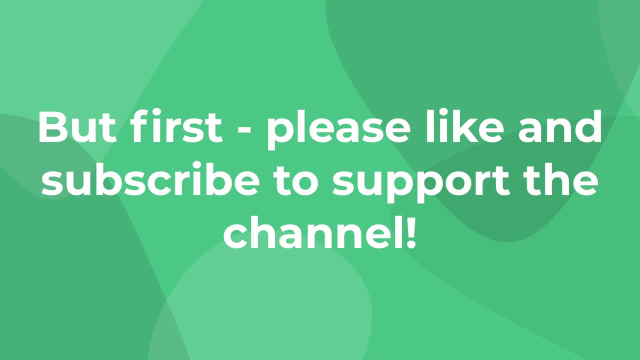 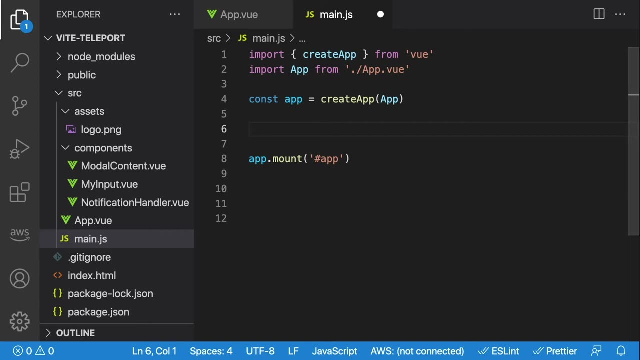 that like button and subscribe to the channel if you haven't. It really helps the video out in the algorithm and allows me to keep creating this free Vue content. So inside our mainjs file or wherever your Vue instance is defined, we just have to use the Vue directive method in Vue 2,. 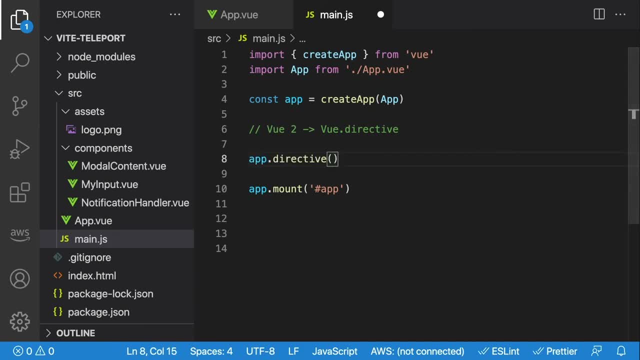 or the app directive method in Vue 3.. But right now, let's create a directive that allows us to manipulate the font size of our component, and it'll be called font size, And from here on out, I'll be implementing the hooks using Vue 3, but you can always. 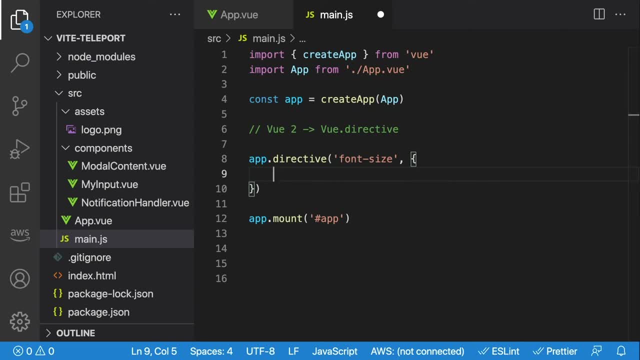 map them to the Vue 2 equivalent. So inside mainjs, once we've created our directive, we want to listen to the before mount hook And once again this will take our l and our binding. To try this out, let's just change the font size of our element to a hardcoded number. 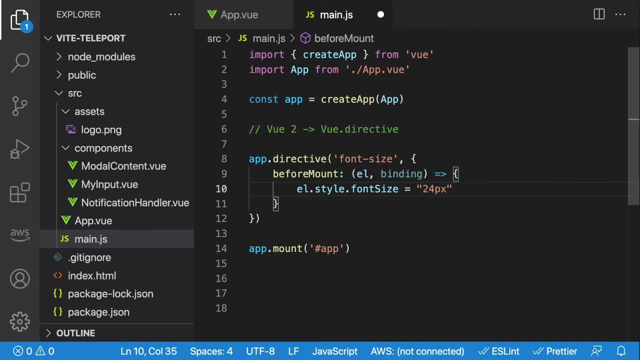 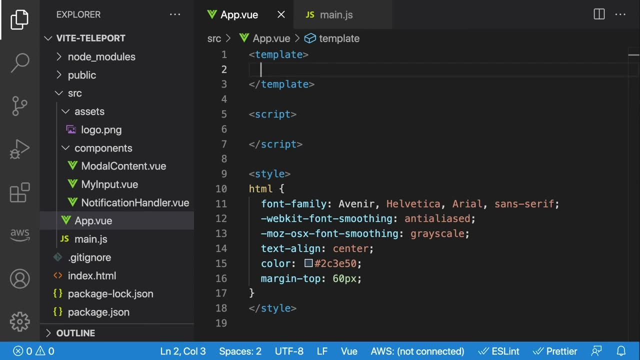 So in here we can just say: lstylefontsize equals, let's say, 24 pixels. So in our appvue component- or whatever component you want, since our directive is installed globally- we can set a normal paragraph and say default font size, And then we can create another one that has our 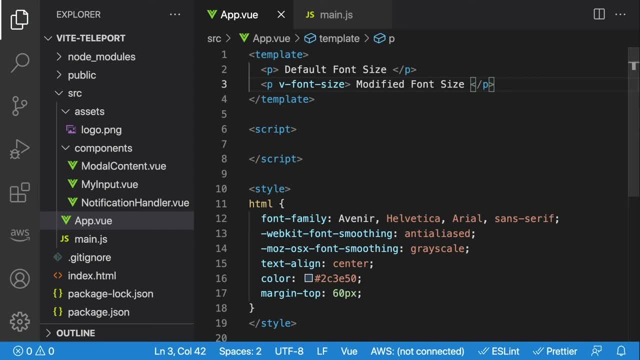 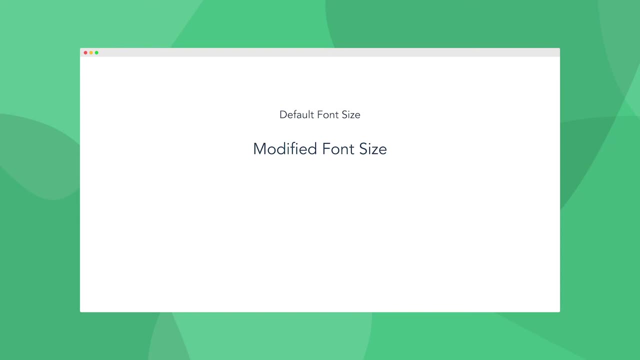 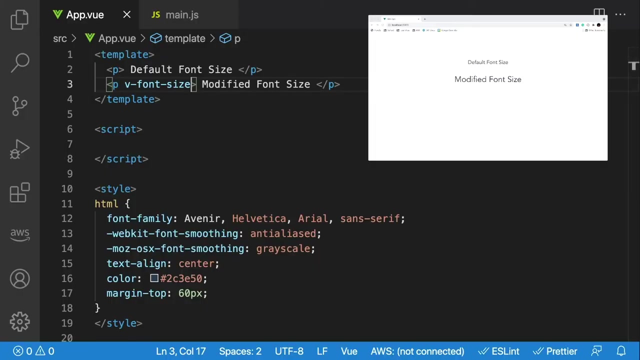 changing the font size with this globally installed directive. Let's work on passing values to our directive. So back in appvue, let's say we want the option to set our font size. we can do that by passing in a JavaScript expression. So here let's just make it something huge, like 100. 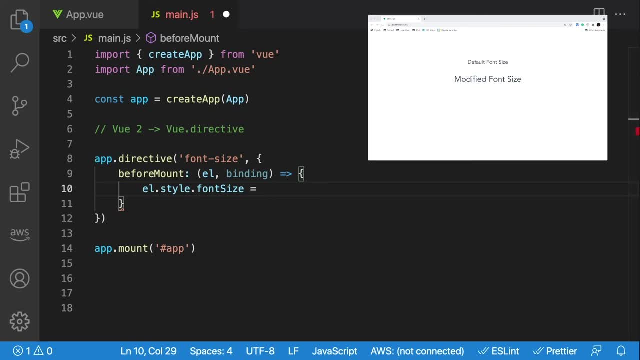 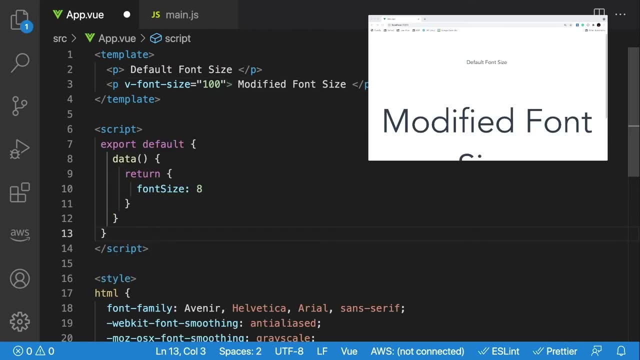 And then inside of our directive. so instead of hard coding it, we can say bindingvalue, And then we have to add our measurements, So pixels. we can also do this by adding a variable. So let's make a variable called font size, pass it in here and also make a button that increases font size. 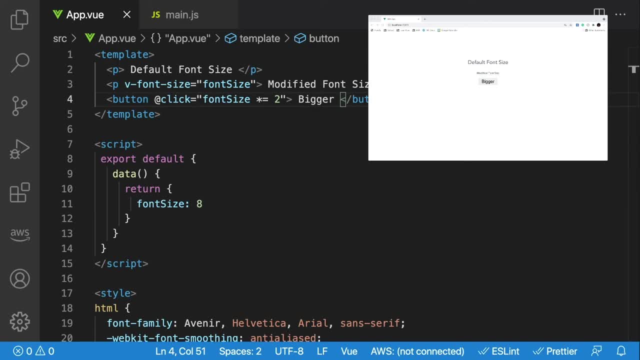 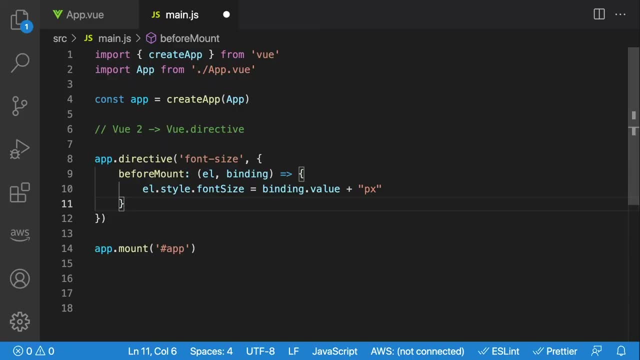 So if we try this out, it displays in the proper size, But when we click nothing happens, And that's because our directive currently isn't set up to handle updating data. But to do this, let's head back over to our directive And we can copy and paste our perform mount hook and then change it. 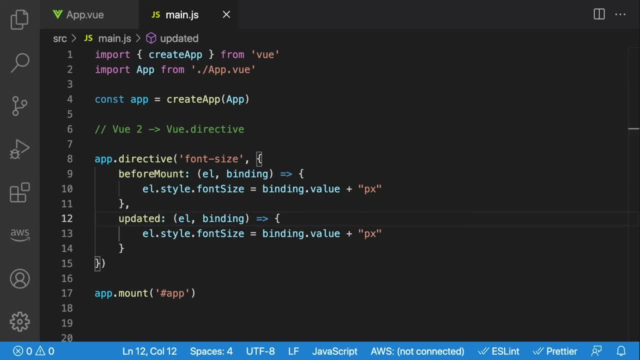 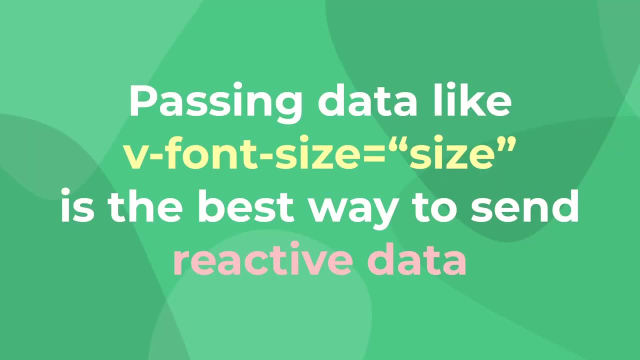 to update it. So this will run whenever the component updates and therefore whenever font size changes. So now, when we click our button, it's all working properly. So passing values is the best way to send reactive data to our directive. So now when we click our button, it's. 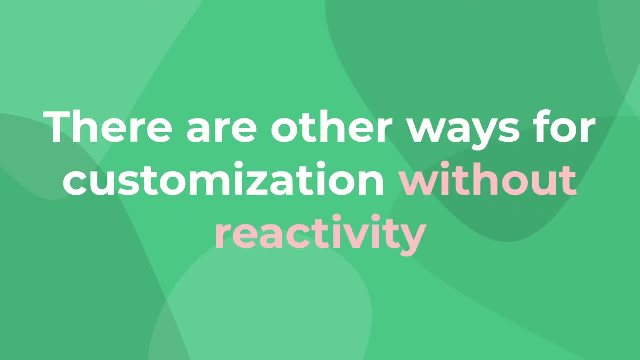 all working properly. So let's head back over to our directive, And if you don't really need any reactivity and just want a way to provide multiple options to your directive- arguments are a great way to do that- Let's start off in our directive. Let's say for our font size that we 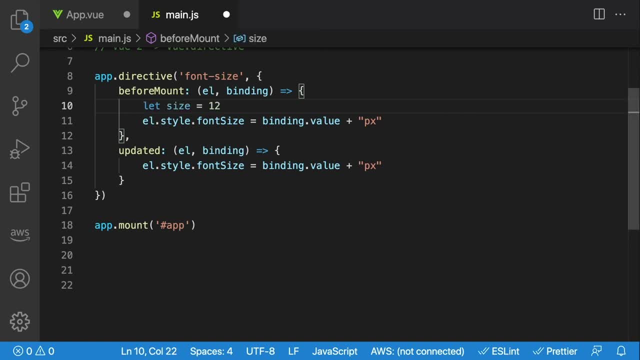 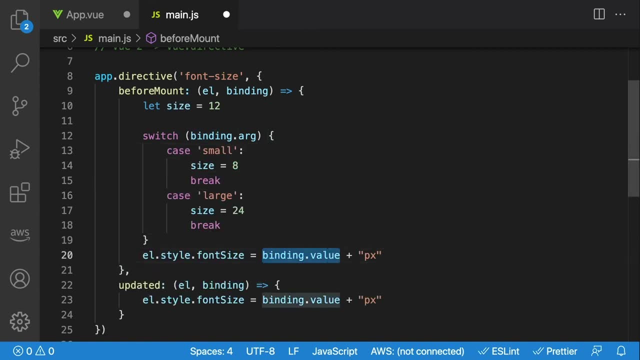 want three different options for small, medium and large. we can set our default size and then switch on this bindingarg value, And if it's small we'll set it to small, If it's large we'll set it to large And otherwise we'll just set it to the default value. And after our switch, let's